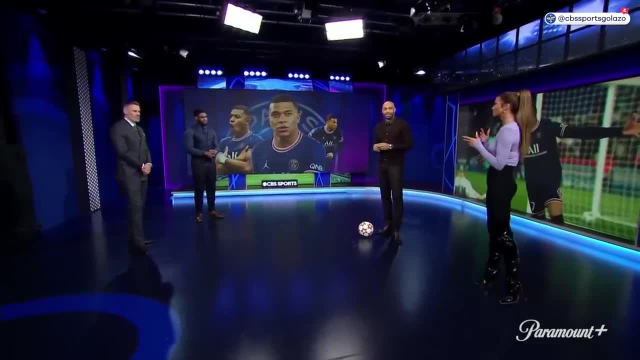 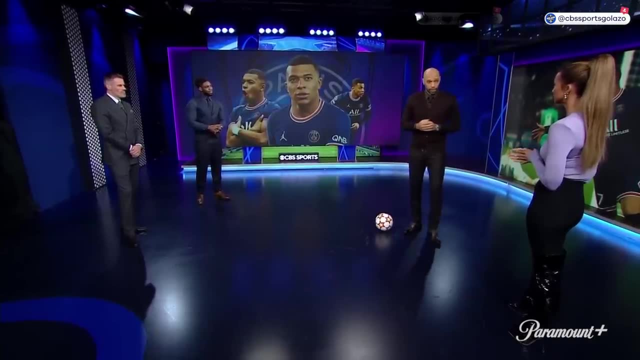 COMPARISONS WITH YOU AND YOUR CAREER. AS WELL CAN YOU BREAK DOWN FOR US WHAT MAKES HIM SO VERY SPECIAL? THAT'S AN EASY ONE, BUT LET'S START WITH THE GOAL THAT HE SCORED THREE WEEKS AGO AGAINST ROYAL MADRID, BECAUSE THAT. 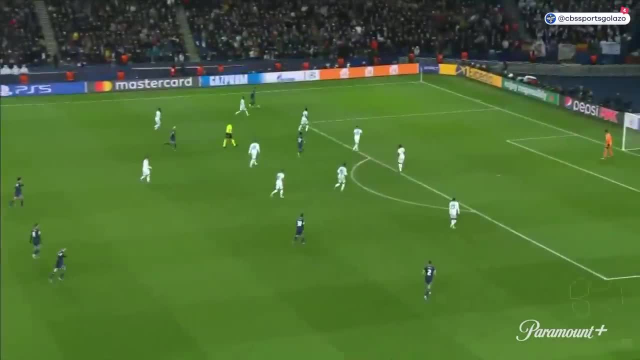 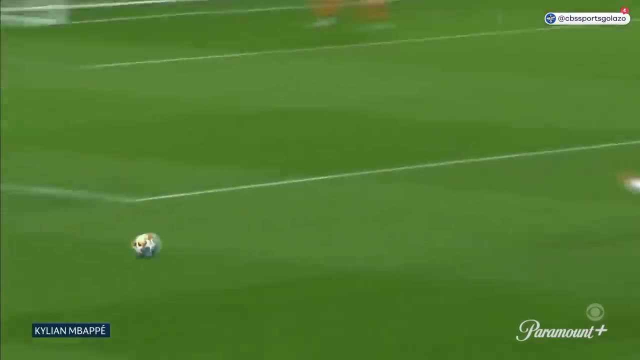 WAS SPECIAL. PEOPLE ALWAYS TALK ABOUT HIS SPEED BUT IT'S NOT ONLY THAT I LIKE THE FIGHTERS. I LIKE THAT HE HAS CONTROL, POWER AND BALANCE WHEN HE IS DRIBBLING. YOU CAN SEE HERE HE IS. 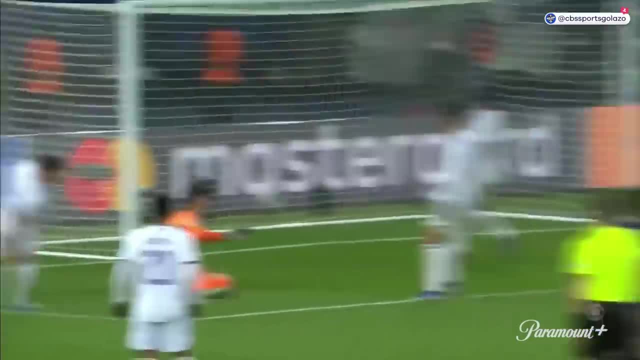 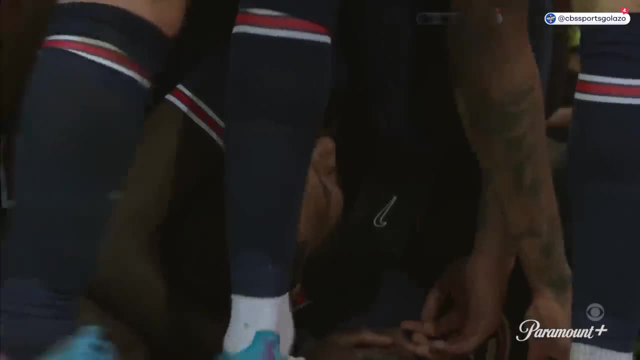 ATTRACTING THE DEFENDER. THEY ARE NAIVE, ENOUGH TO OPEN THAT WINDOW, AND IF YOU OPEN THE WINDOW, HE WILL STEP INTO YOUR HOUSE AND SCORE: HOW DOES THIS WORK? YOU CAN SEE EVERY TIME IT'S LIKE GOING SLOWLY, PUSHING THE. 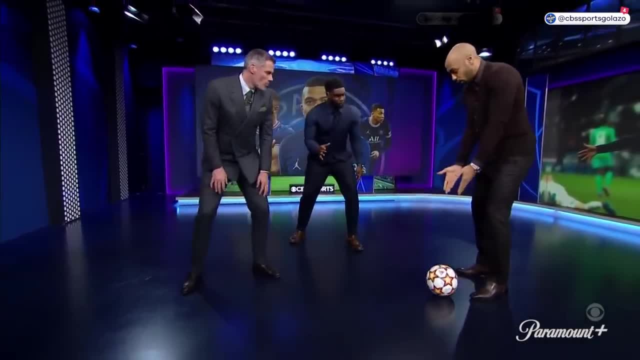 BALL ON EVERY STEP ALMOST HE IS TRYING TO SEE IF HE IS GOING TO BUY THIS. I NEVER UNDERSTOOD THAT WITH THE DEFENDER. WHY? BECAUSE YOU DEFEND THE BALL, OBVIOUSLY, AND THE GOAL BUT. 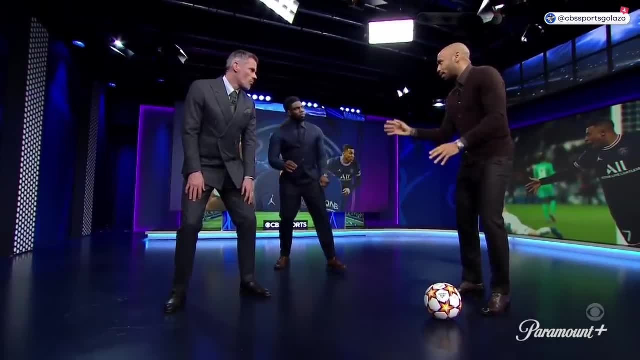 YOU ALWAYS, AT ONE POINT, WANT TO COME AND GET IT, OR YOU ARE OVERSTEPPING SOMEWHERE. WE DON'T WANT TO GIVE YOU TIME TO THINK ABOUT WHERE YOU ARE GOING TO GO NEXT WITH THE BALL, SO WE ARE TRYING TO GET THERE AS SOON AS POSSIBLE. 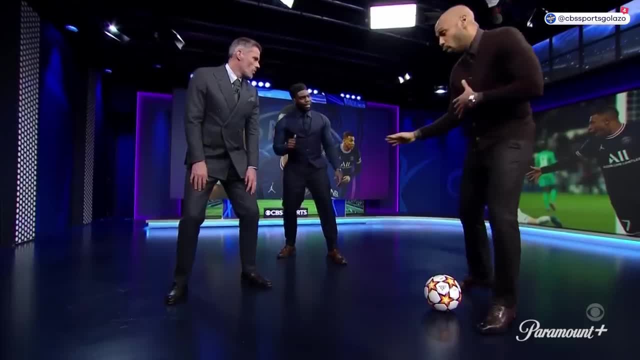 THAT'S EXACTLY WHAT THEY DID. THEY OPENED THAT LITTLE WINDOW. HE WENT IN BECAUSE HE HAS THE TECHNIC, NOT ONLY THE SPEED. SO HE GOES IN, GENERATES POWER ON HIS RIGHT FOOT, ON HIS LEFT. 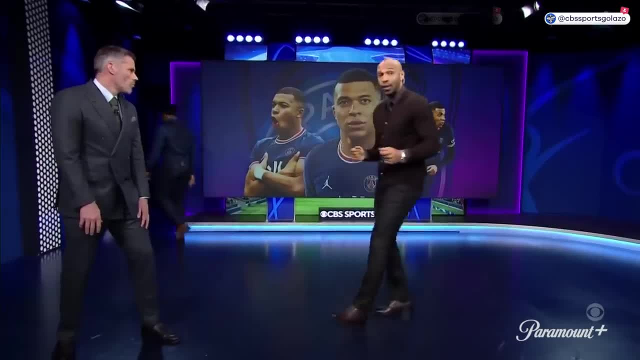 FOOT AND HE HAS THE COMPOSURE TO FINISH IT AT THE END OF A GAME IN THE CHAMPIONS LEAGUE. THAT'S NOT SO. HE'S JUST WAITING FOR THAT TO OPEN UP. IT IS BECAUSE, IF YOU THINK ABOUT IT, HE'S DOING THIS. 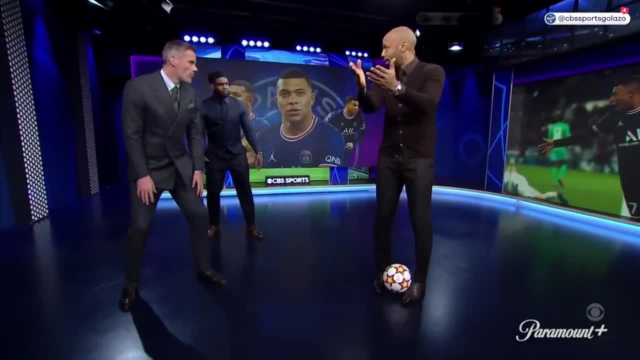 HE'S DOING THIS. HE'S DOING THIS. WHERE CAN HE GO? THERE? THE GOAL IS THERE, BUT IF YOU OPEN THAT WINDOW, HE'S WAITING. ARE YOU MOVING? IF YOU'RE MOVING, I'M GOING. 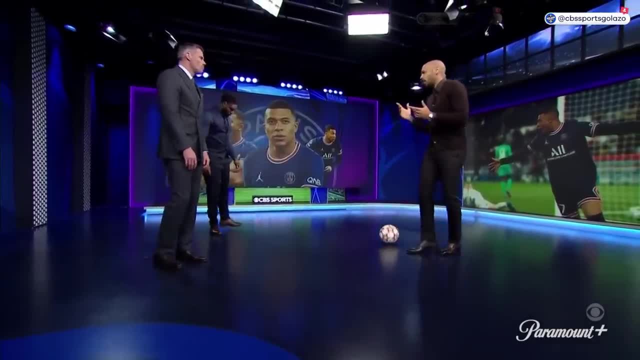 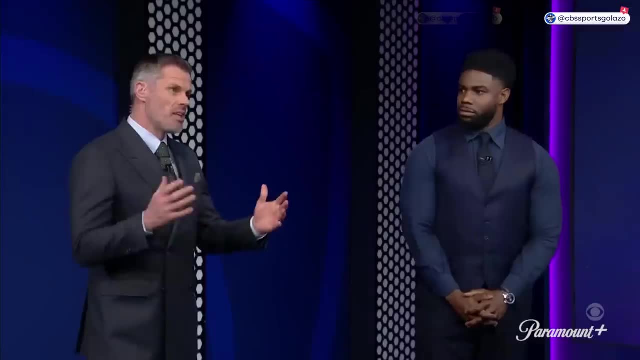 THIS IS WHAT HE DID, AND HE DOES THAT TO THE T, AND I LIKE THE WAY HE THINKS ABOUT IT, BECAUSE HE THINKS ABOUT HOW HE CAN SCORE GOALS. IT DOESN'T JUST HAPPEN LIKE THAT. THAT'S IN TIGHT SPACES AND IT IS WHAT MAKES EMBAPE. SO 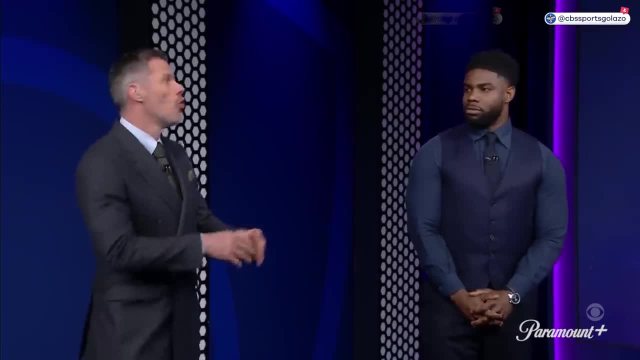 SPECIFIC. HE CAN DO IT IN TIGHT SPACES OR HUGE SPACES. WE'VE GOT A CLIP HERE FROM THE CHAMPIONS LEAGUE THIS SEASON, AS WELL WHERE HE'S GOT SPACE AND IS THIS WHERE HE'S AT HIS. 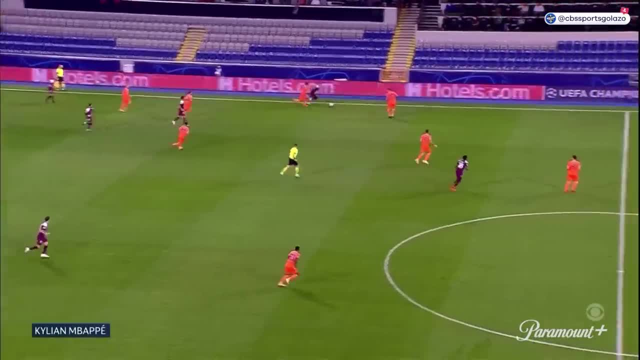 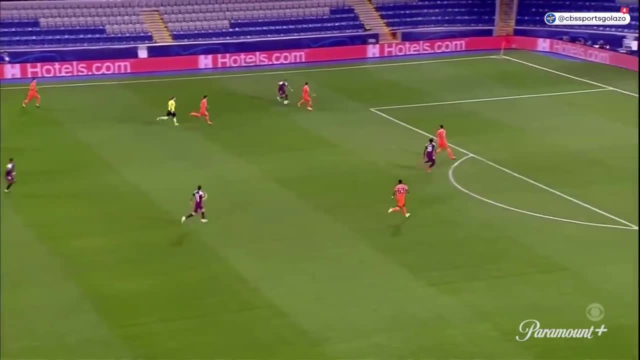 BEST. IT IS FIRST AND FOREMOST. SAME THING POWER TECHNIQUE. NOW, IF YOU GIVE HIM THAT YOU'RE NEVER GOING TO SEE HIM AGAIN, THE STRENGTH THAT HE HAS IN HIS LEG TO BE ABLE TO DO THAT WITH THE BALL AT YOUR FEET DANCING. 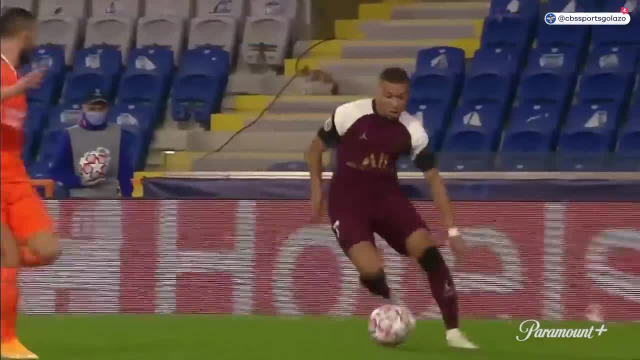 AROUND WITH THE DEFENDER, AND THEN YOU CAN SEE HERE. HE LOST A BIT OF HIS BALANCE. THAT'S WHY HE COULDN'T FINISH IT. AND IN AND AROUND, YOU WILL SEE HERE. THIS IS WHAT HE'S. 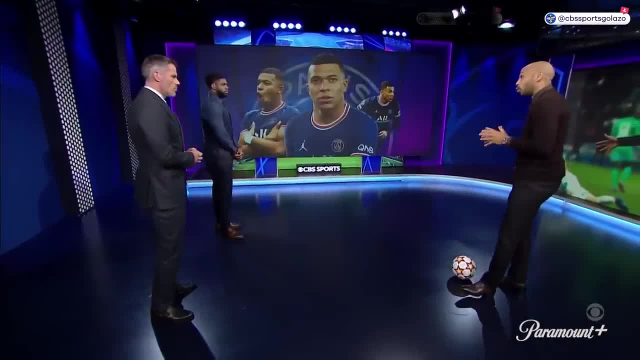 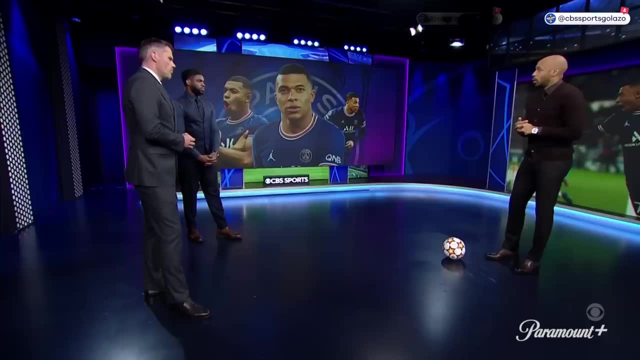 DOING. THIS IS WHY IT'S SO DIFFICULT TO KEEP YOUR COMPOSURE AND YOUR BALANCE WHEN YOU'RE RUNNING WITH THE BALL AT FULL SPEED. WHAT DO YOU SEE FROM YOUR GAME IN KILLING AN EMBAPES? WELL, WITH ALL HUMILITY, BECAUSE THIS GUY IS JUST A. 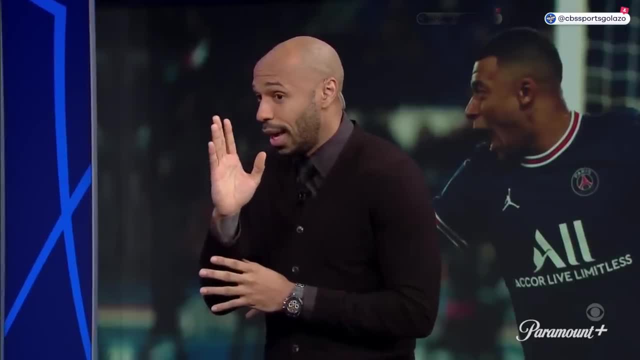 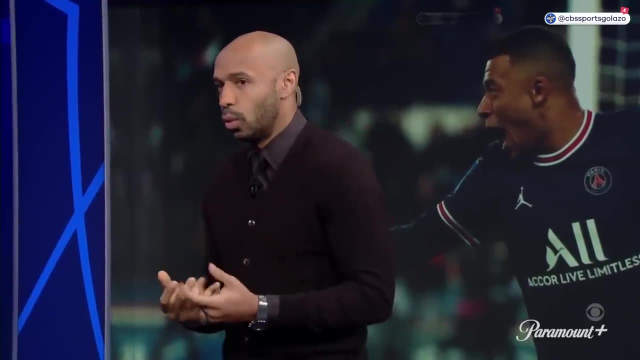 FREAK, BUT THE WAY HE COULD. SEE A GOAL AND THINK ABOUT IT. SEE THE PATH AND EXECUTE IT. SOMETIME YOU SEE A 1 V 11, EVERYONE WILL TELL YOU: WOW, IT'S 11 PLAYERS TO BEAT. 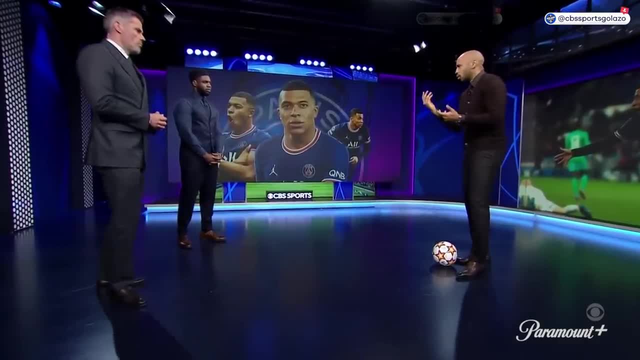 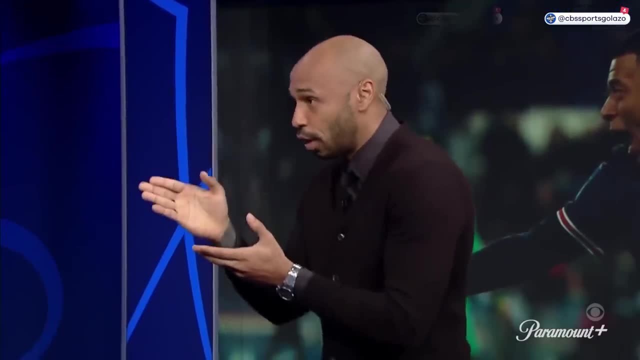 IT'S NOT 11 PLAYERS TO BEAT, IT'S THE LINE. DO YOU KNOW WHAT I MEAN? AND I USED TO THINK LIKE THAT: FIRST AND FOREMOST, WIN YOUR 1 V 1.. THEN YOU WOULD HAVE ANOTHER. 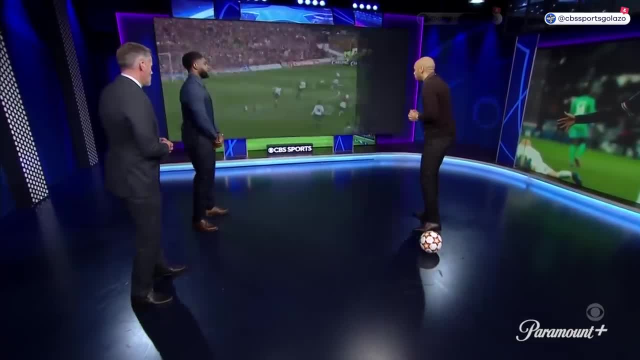 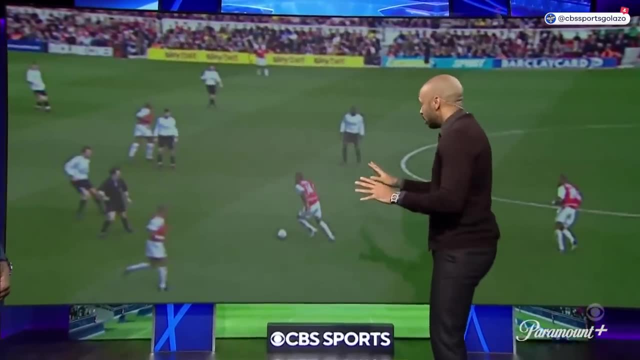 AND THEN YOU WILL SEE THE GOAL KEEPER LOOK AT THE GOAL I SCORED AGAINST LIVERPOOL. I DON'T KNOW WHY. I'M THERE, BY THE WAY, BUT I'M THERE. I WISH YOU WINS. 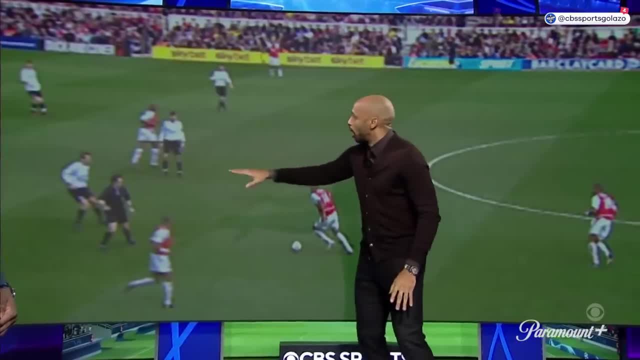 THIS IS THE PICTURE: EMILESKI OWEN IS UP FRONT AND YOU HAVE TWO LINES OF FOUR. AT THAT MOMENT, IT'S A 1 V. OKAY, IT'S A 1 V 9, BECAUSE THE GOAL KEEPER IS THERE. 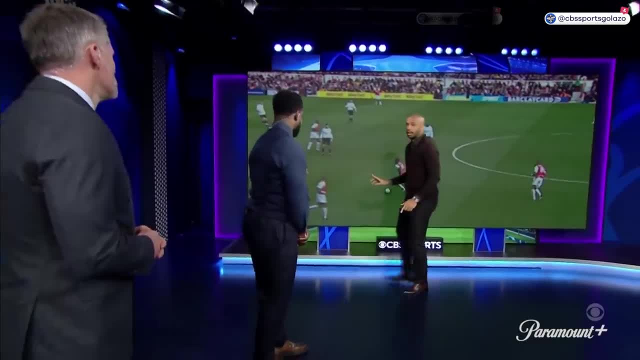 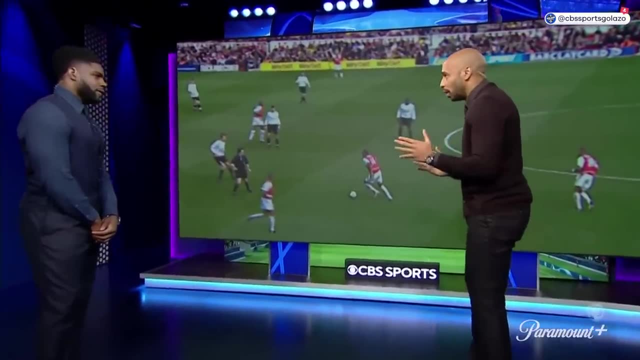 ALL I'M THINKING IS: IT'S A 1 V 1 WITH DIDI AMAN, AND I KNOW, AT A PARTICULAR MOMENT, IF I PUSH THE BALL, WELL, I SHOULD BEAT HIM, BUT YOU HAVE TO BE EQUIPPED. THAT'S WHY I TALK ABOUT TECHNIQUE AND CONTROL WHILE YOU'RE RUNNING. 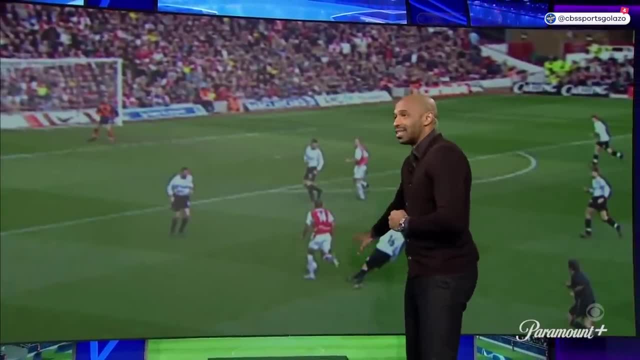 I DIDN'T PUSH THE BALL TOO WELL THERE. I HAD TO PUSH IT AGAIN NOW. I KNOW HE FAILED HE'S OUT. I DON'T HAVE TO LOOK BEHIND ME. IT'S OVER NOW. 1 V, 1 AGAIN. 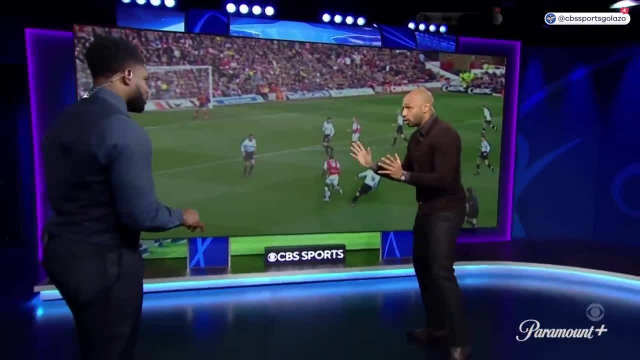 AND I NEED TO MAKE THEM BELIEVE ALL OF THEM, AND MORE SO, JAMIE THAT I'M GOING TO SHOOT WITH MY RIGHT FOOT TO BE ABLE TO GO INTO THE LITTLE SPACE THAT THEY'RE GOING TO OPEN. 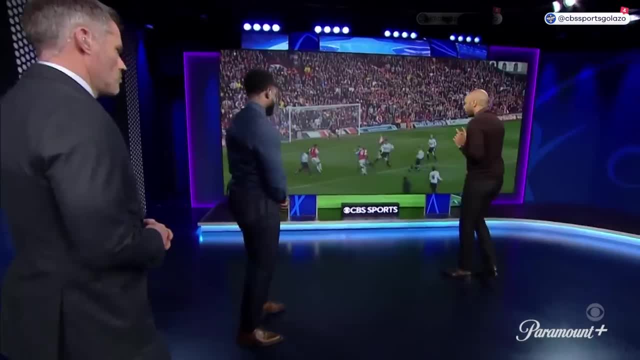 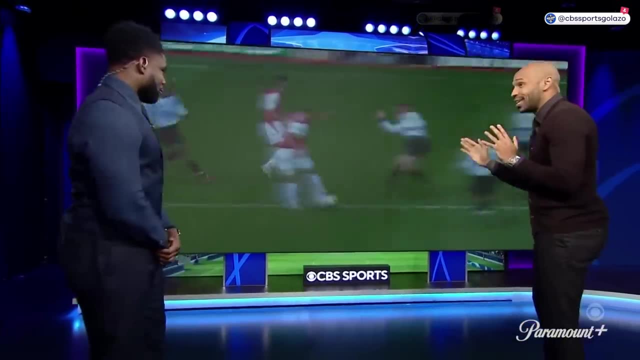 IF THEY BELIEVE IN IT. BUT WHAT IF HE WAS TO TAKE A STEP? WELL, IF HE DID TAKE A STEP, I WAS DEAD, BUT HE DIDN'T. THIS IS WHAT I THOUGHT AT THE TIME WHEN I DID IT. 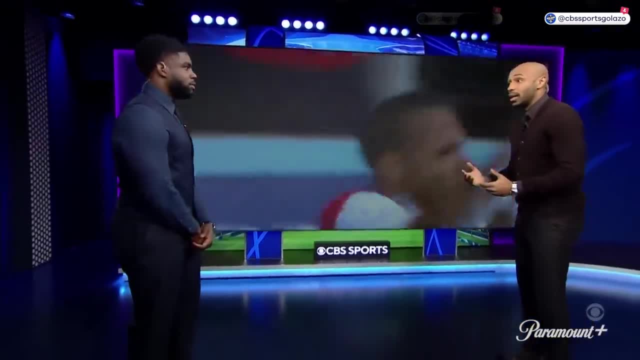 YOU CAN'T GO THERE AND GO. WHAT AM I DOING NOW, BECAUSE IT'S TOO LATE. I THOUGHT ABOUT IT WHEN I PASSED DIDI AMAN, WHEN I PASSED DIDI AMAN, THEN I PASSED JAMIE. 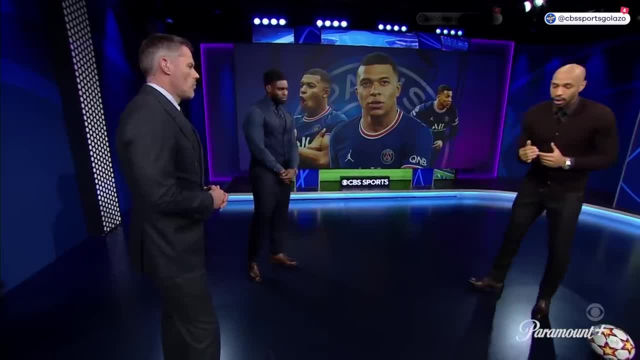 THEN I WENT INSIDE, I RECOMPOSED MYSELF TO FINISH WITH DUDEK. THAT'S WHY I THINK KILLIAN EMBAPE ALSO HAS. HE CAN SEE THE PATH AND HAS THE ATTRIBUTE TO EXECUTE IT. THAT'S VERY IMPORTANT TOO. 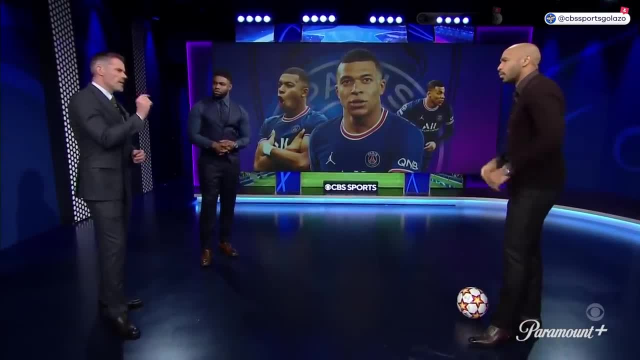 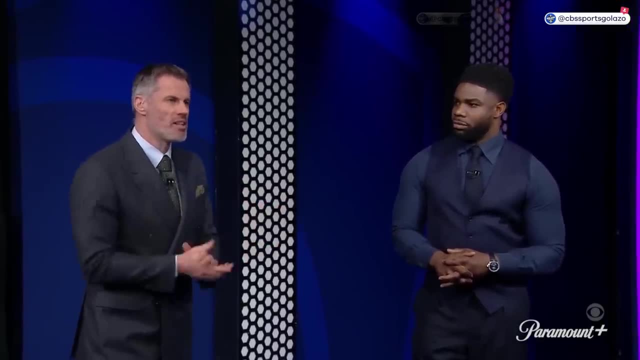 BUT WHAT I THINK YOU HAD, AND KILLIAN EMBAPE CERTAINLY HAS, IS THEY PUT FEAR IN DEFENDERS. NOW I'M LOOKING AT THAT AND THAT IS EMBARRASSING- DEFENDING FROM MYSELF. 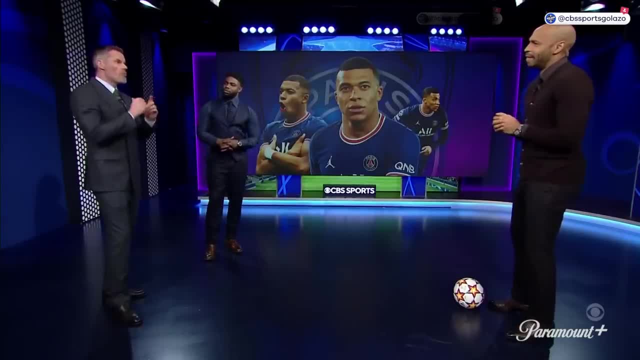 BUT I KNOW THE EFFECT YOU USED TO HAVE ON ME, CERTAINLY FOR THE THREE OR FOUR-YEAR PERIOD WHEN I WAS PLAYING AGAINST YOU. I DON'T THINK I PLAYED THE WAY I WOULD AGAINST SOMEBODY ELSE. 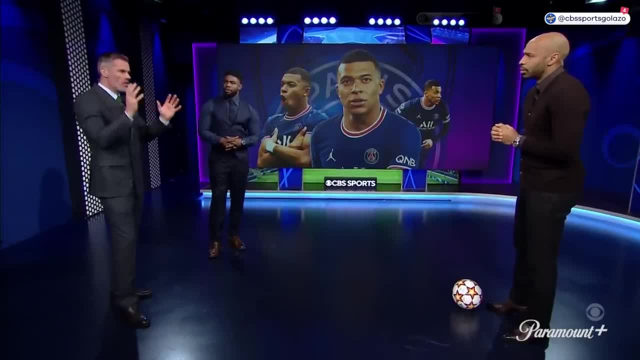 BECAUSE IT WAS YOU, AND I THINK KILLIAN EMBAPE AND THE GREAT PLAYERS HAVE THAT EFFECT ON DEFENDERS. DID YOU FEEL LIKE YOURSELF- NOT JUST AGAINST ME OR OTHER DEFENDERS- WHEN YOU WERE AT YOUR PRIME? 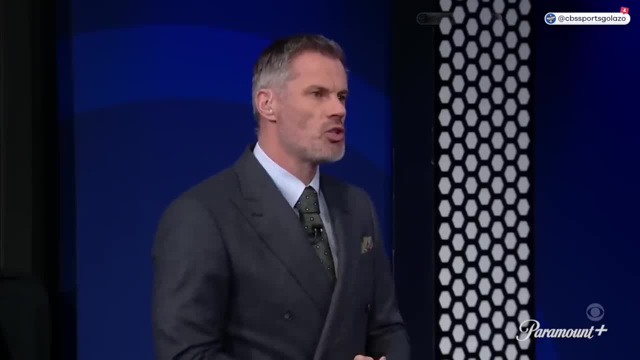 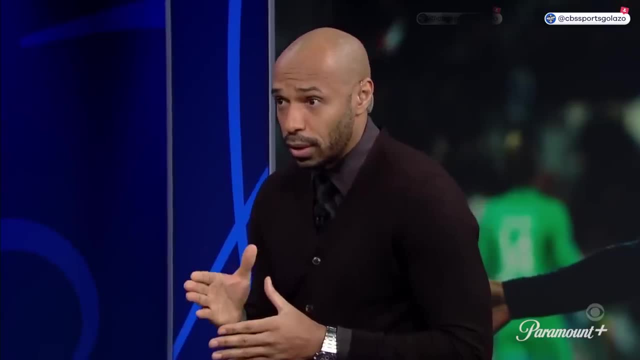 THAT THERE WAS FEAR IN THEIR EYES WHEN THEY WERE COMING AGAINST YOU. YES, BECAUSE SPEED DOES MAKE PEOPLE SCARED YOU UNSTALL FEAR INTO DEFENDERS, BUT ALSO AT THE BEGINNING OF THE GAME. 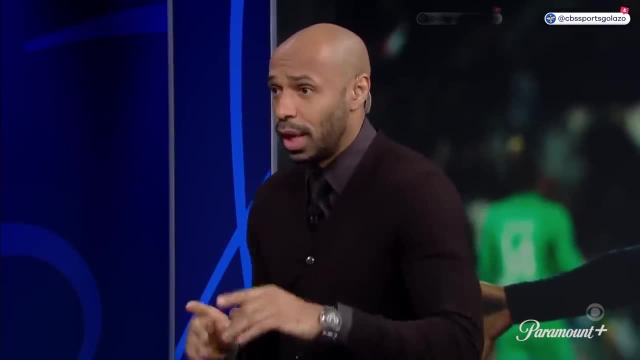 I WAS ALWAYS GOING TO GIVE YOU THAT FIVE RUNS FOR NO REASON BEHIND TO LET YOU KNOW. OH, I'M FASTER, THAN YOU, SO STAY THERE SO I CAN GET MY BALL AND MAYBE DO THAT. 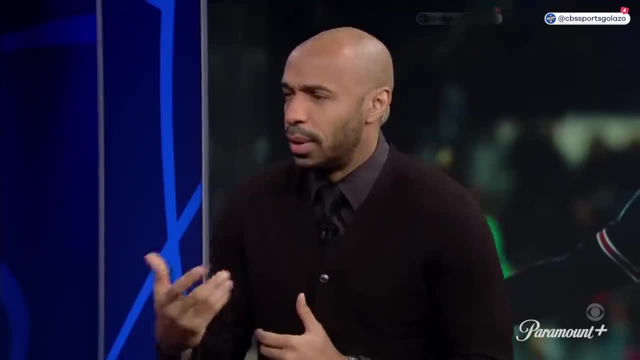 BUT ALSO THERE'S SOMETHING. THAT'S IMPORTANT. YOU NEED TO HAVE A LOT OF WEAPONS, BECAUSE IF IT WAS ONLY ABOUT SPEED, YOU WOULDN'T HAVE BEEN SCARED, BECAUSE THERE WAS A LOT OF GUYS. 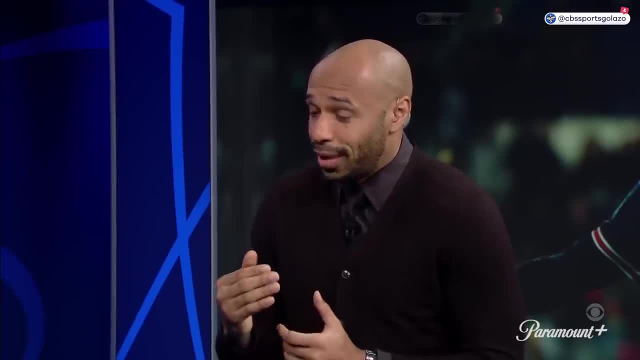 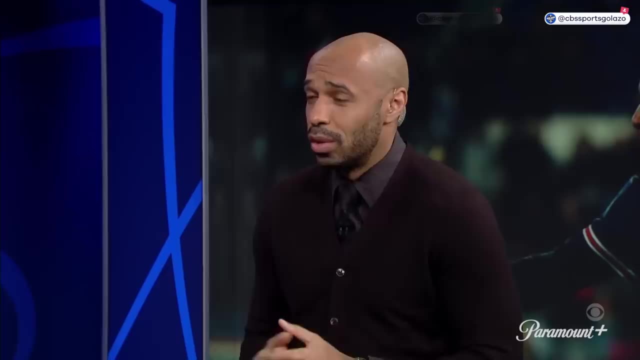 THAT WERE FAST IN THE LEAGUE AT THE TIME, BUT IF YOU HAD LIKE, I MENTIONED CONTROL, SPEED, ACCURACY, BALANCE, LEFT FOOT, RIGHT FOOT. IT'S ALMOST DIFFICULT, ALMOST VIRTUALLY. 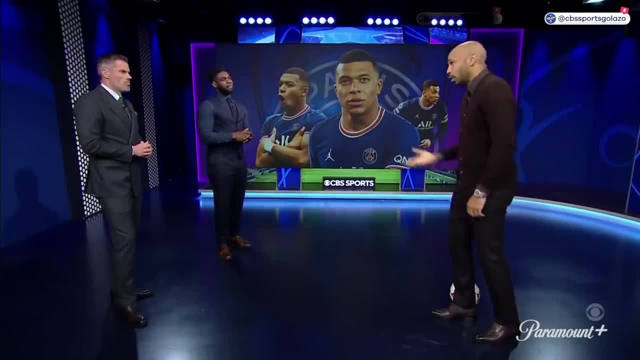 I WOULD SAY IMPOSSIBLE TO DEFEND, BUT LIKE. I WOULD LIKE TO SAY: YOU, GUYS, TOP ME MORE THAN I PASS YOU. ALL I NEED IS ONE. SO PLAYERS LIKE EMBAPE MIGHT HAVE LEARNED. 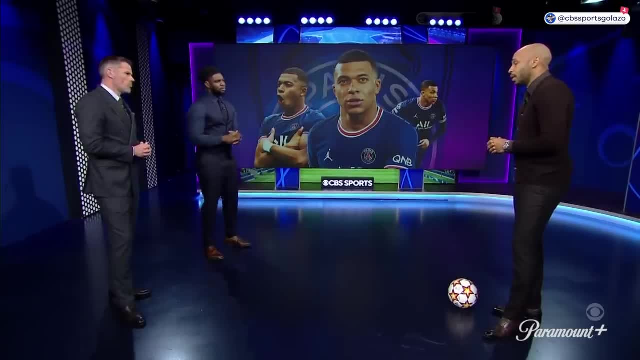 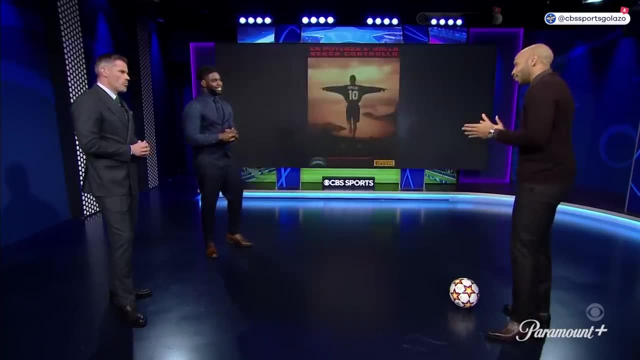 THE WAY THEY MOVE FROM YOU. WHERE DID YOU LEARN IT FROM? WELL? THERE WAS THREE GUYS: GEORGE, WEAH, ROMARIO AND THE ONE AND ONLY OUR NINE, RONALDO BRAZILIAN RONALDO. 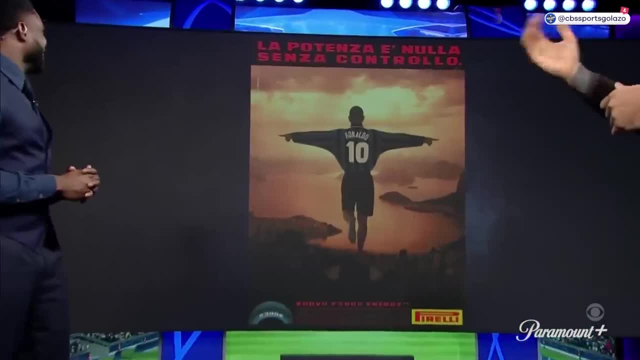 WHAT DOES THIS MEAN HERE? WELL, YOU PLAYED IN ITALY. WELL, TELL ME, PLEASE. YOU PLAYED IN ITALY, WELL, I DIDN'T GET THE NEXT STAGE OF THE GRABBER. 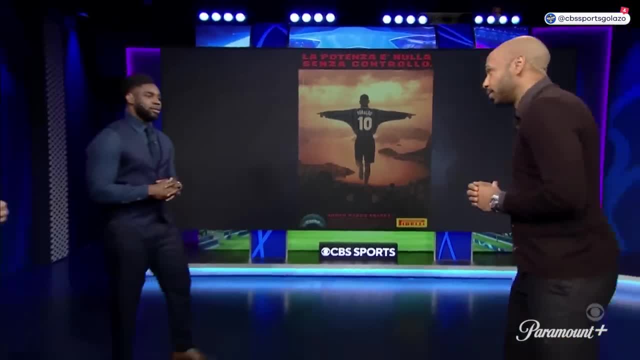 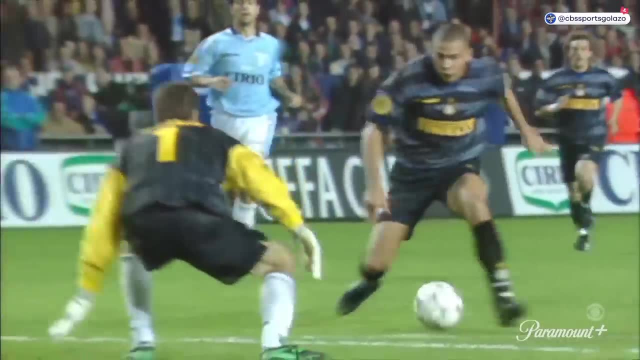 POWER IS NOTHING WITHOUT CONTROL, OK, AND HE HAD THAT IN ABUNDANCE, I MEAN, I UNTIL, I MEAN I'M LOOKING AT IT AND I DON'T KNOW HOW HE DIDN'T BREAK HIS LEG. 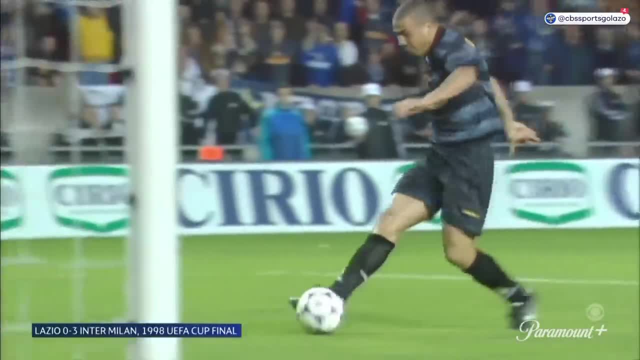 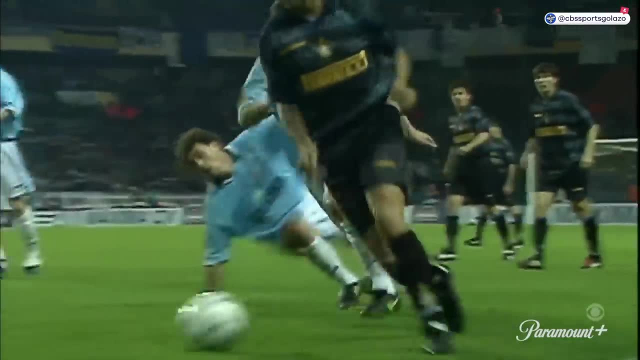 THE POWER THAT IT GENERATES, TO GO ONE WAY TO THE OTHER, TO CHANGE- AND HE COULD DO THAT, BY THE WAY- EVERYWHERE ON THE FIELD. TAKE THE BALL, AND WE CAN SEE HERE. OOPS, NO, THE QUALITY THAT RONALDO HAD. 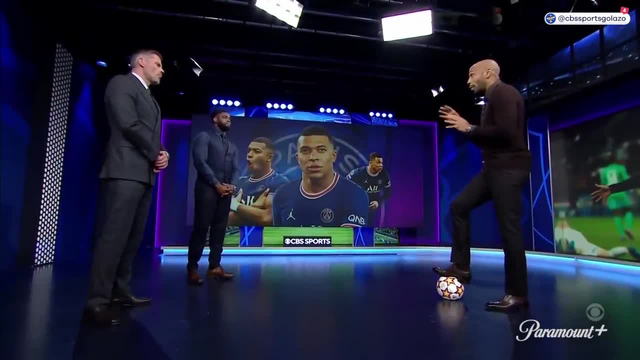 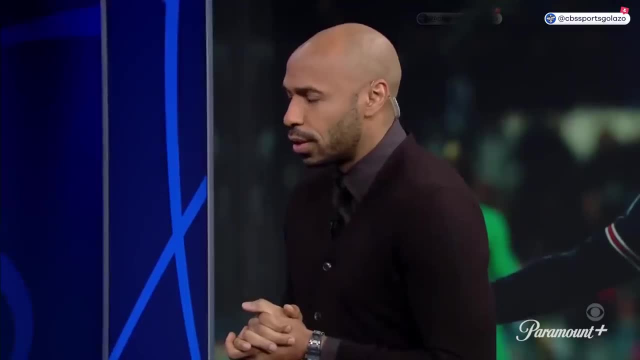 WAS JUST, FOR ME, THE BEST THAT I'VE SEEN, WHEN YOU COMBINE ALL THE WORDS AND ALL THE ADJECTIVES THAT I JUST MENTIONED BEFORE ABOUT EMBAPE. HE WAS JUST OUT OF THIS WORLD, SO YEAH. 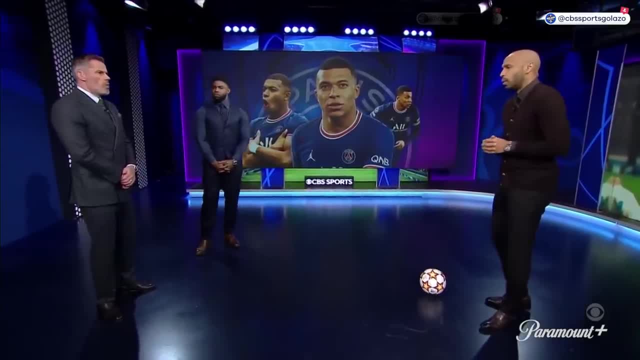 HE'S THE GUY THAT INSPIRED ME A LOT IN TERMS OF DOING THAT WITH THE BALL. IS THERE ANYTHING IN EMBAPE'S GAME IN THE LAST YEAR OR TWO THAT YOU THINK'S TAKING HIM TO THAT NEXT LEVEL NOW? 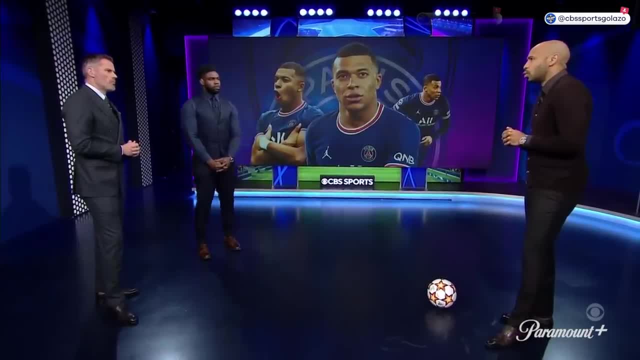 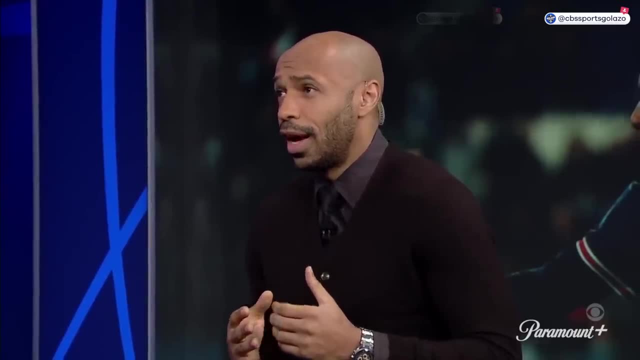 HE FINISHES BETTER. HE USED TO DO A LOT OF SKILLS SOMETIME AND HE UNDERSTOOD IN THE PAST YEAR AND A HALF, IF I CAN SAY, BECAUSE HE'S BEEN MAGNIFICENT SINCE. 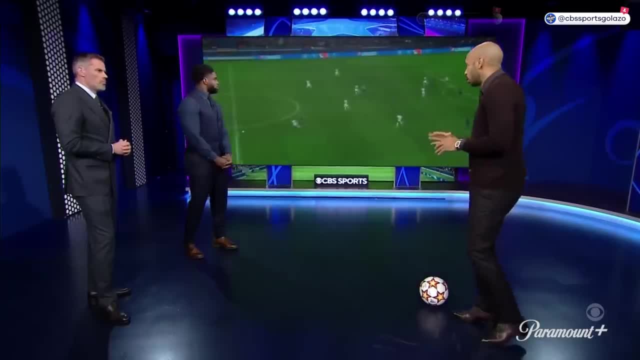 THAT NOW. HE NEEDS TO BE EFFICIENT, MORE OFTEN THAN NOT FINISH, FINISH. HE HAS TO STOP GOING AROUND AND TRYING TO PLEASE THE CROWD. YOU CAN PLEASE THE CROWD BY DOING THIS. 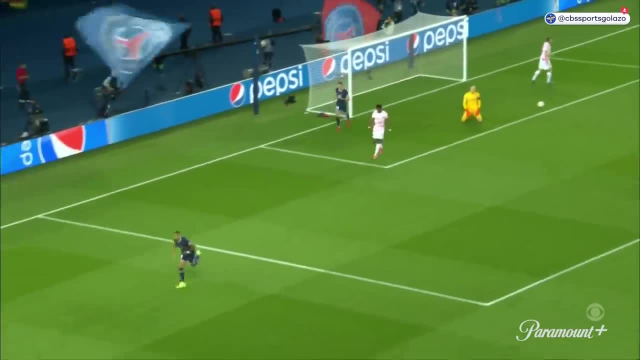 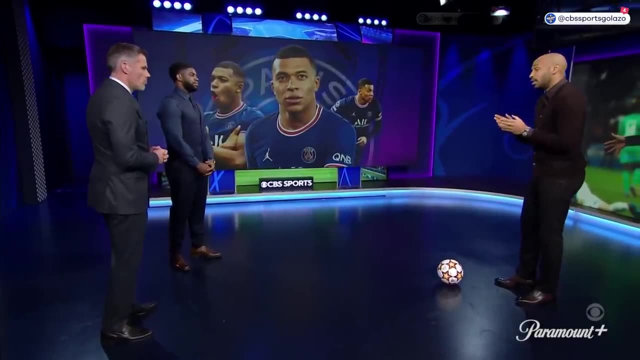 AND THIS IS SOMETHING THAT HE DID RECENTLY. HE USED TO LIKE TO CURVE THE BALL, SHIFT THE BALL IN AND CURVE IT INTO THE TOP CORNER. NOW HE'S GIVING DEFENDERS- ANOTHER PROBLEM. 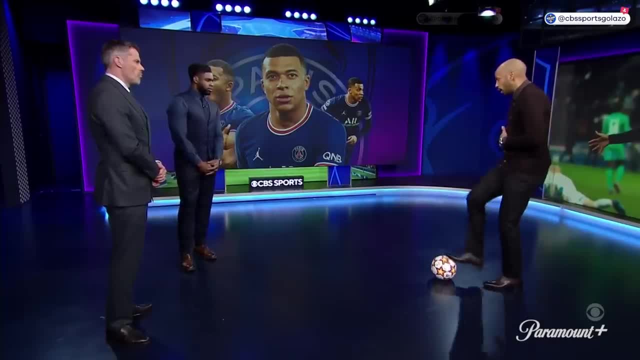 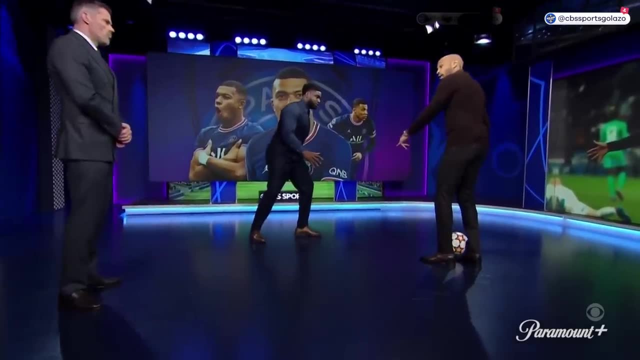 ANOTHER WEAPON: NOW, WHEN HE PUSHES THE BALL HERE, HE'S WAITING FOR YOU TO OPEN YOUR LEG, OBVIOUSLY, WHEN YOU SHIFT IT, TO HIT IT THROUGH YOUR LEGS. SO NOW HE CAN BEND OR HE CAN HIT IT THROUGH YOUR LEGS. 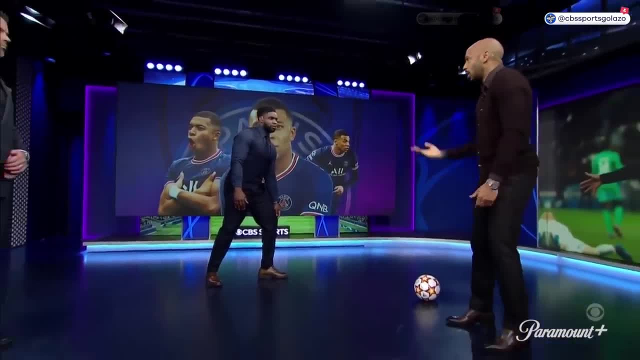 SO NOW, YOU DON'T EVEN KNOW IF YOU HAVE TO PUT YOUR LEG UP OR NOT, EVEN KNOW IF YOU HAVE TO PUT YOUR LEG UP OR NOT. SO THIS IS WHY I THINK THIS GUY IS CLEVER, BECAUSE HE DOESN'T STAY ONLY.